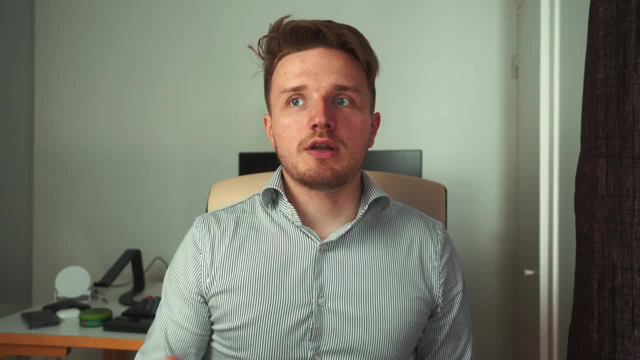 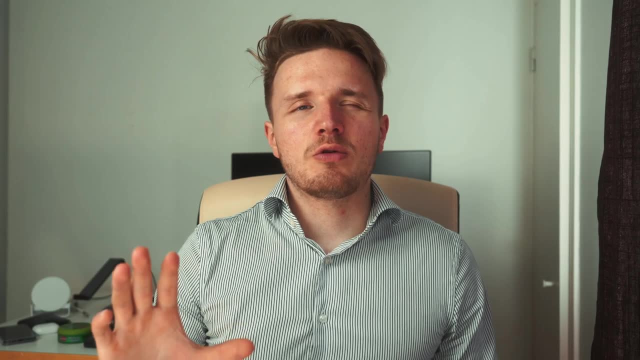 and find my discount code for 10% off their subscription. If you want to just do the Python course, that's absolutely fine. You can probably finish it in like one to two weeks or three weeks, depending on how many hours you're able to put in, and then you can just unsubscribe after that. 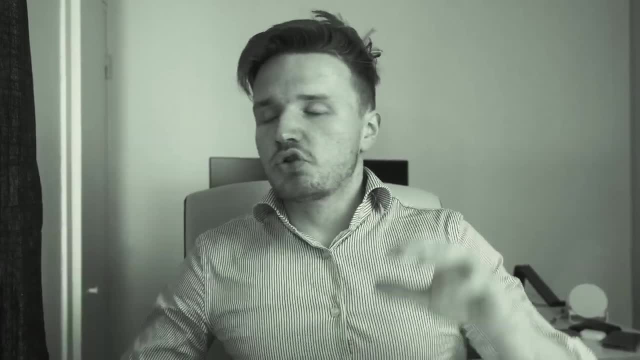 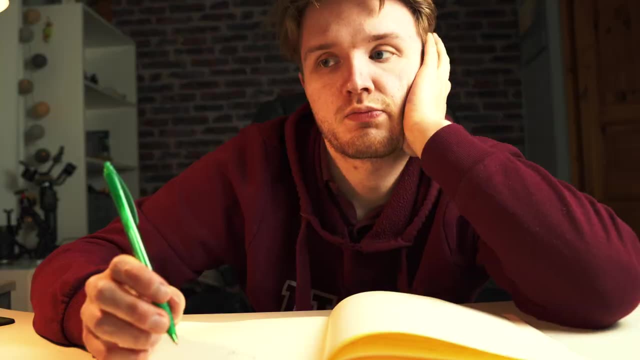 And you might already be saying that doing courses isn't enough, You shouldn't just do tutorials, blah, blah, blah, And I'll be the first one to agree. I'll be the first one to agree that, if you want to learn a programming language, the biggest mistake that people make is that they 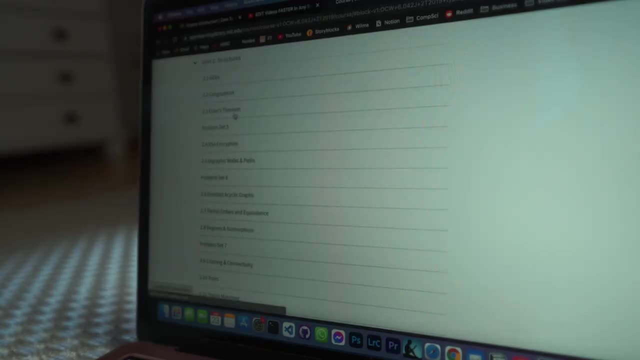 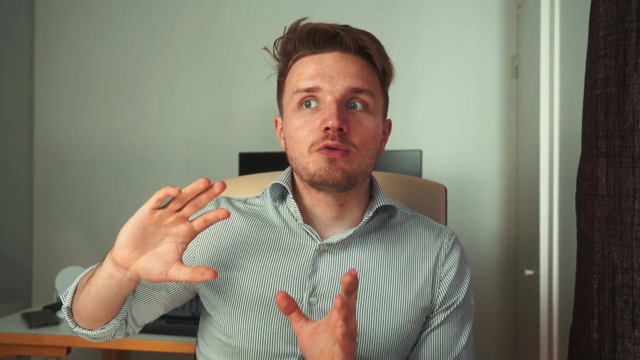 just focus on tutorials, they just focus on doing some course and they just leave it at that. That is not how you actually master a language, and I'll talk about the other things that you need to do further on in this video, But to get started with you absolutely should start. 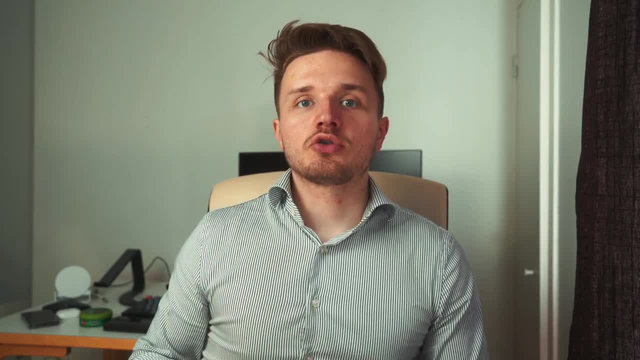 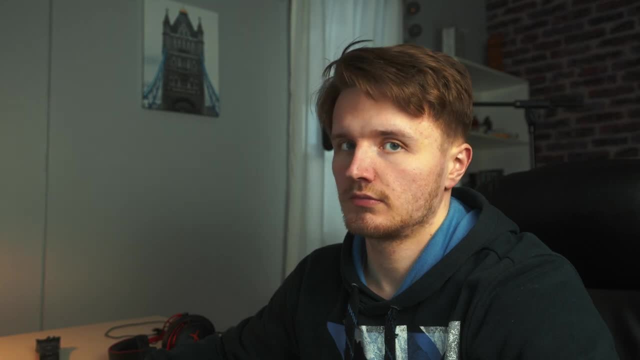 with some course, with some tutorials to get you acquainted with the language, to get you acquainted with the basics, because you can't really start building anything before you are even familiar with the language. But that is when we get to steps two, three and four. 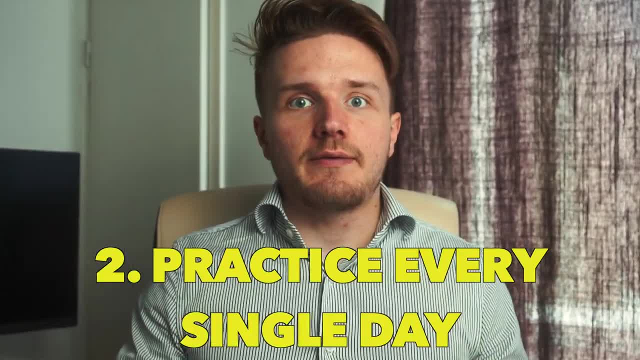 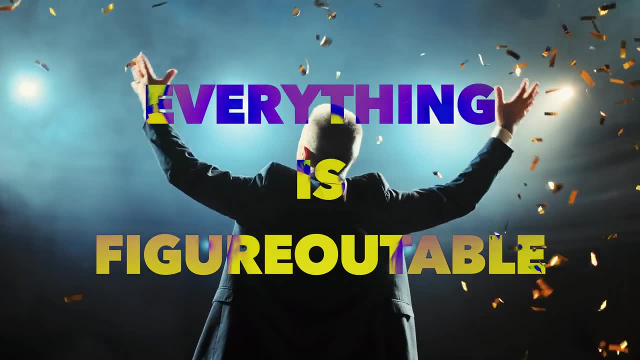 Which I'll talk about next Second. you need to practice every single day. What you need to understand is that coding, Python, any language or any other skill, everything is learnable, everything is figureoutable. But in order to learn these kinds of skills, all we have to do 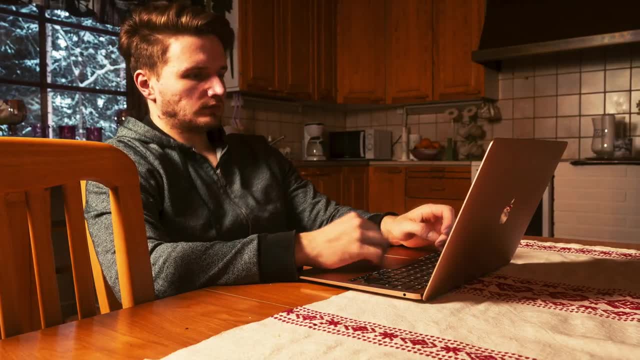 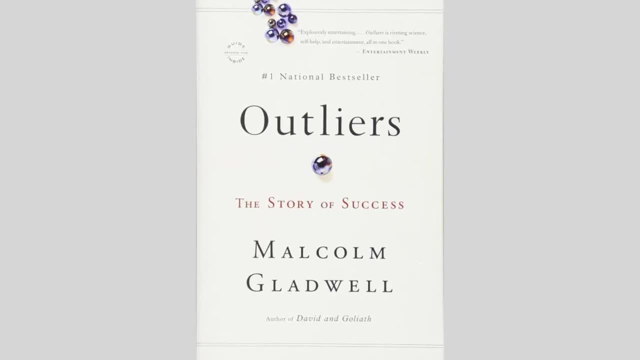 is just put in the practice and be consistent with it. I cannot stress enough how important this is. There's a great book on this topic called Outliers by Malcolm Gladwell, where he essentially introduces this idea of the 10,000 hour rule, where, if you want to master any kind 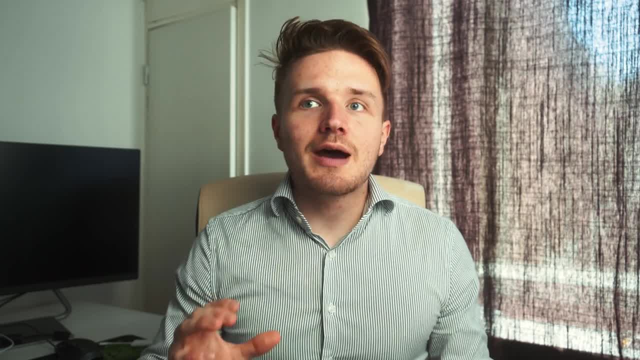 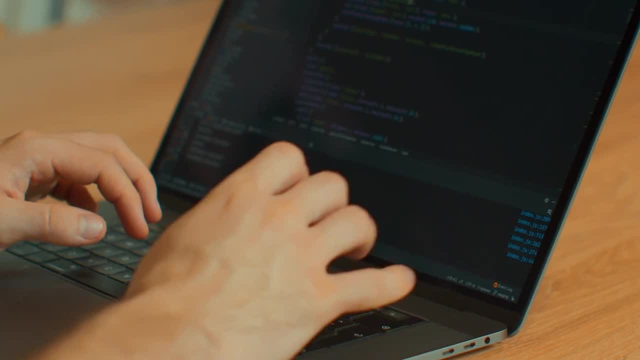 of skill. you need to practice it for 10,000 hours cumulatively before you can really be great at it. So if you need to do 10,000 hours, it's not enough to just do one hour a week. That. 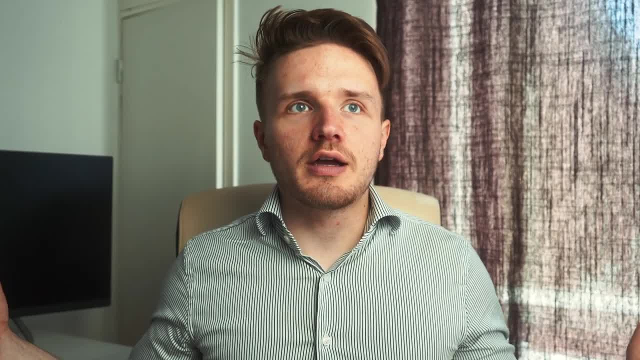 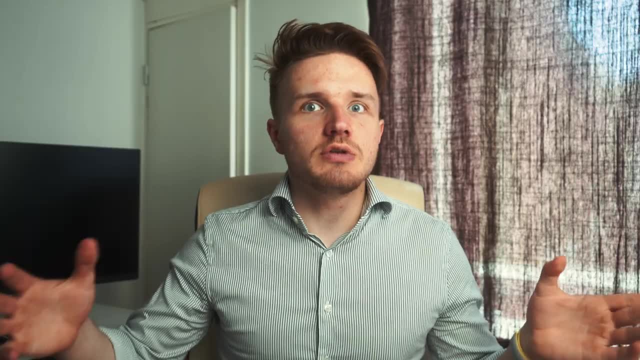 would take like 10,000 weeks, which is like probably longer than our entire lifetimes. So you need to be consistent and you need to put in the work every day. There's obviously no set amount of hours that you need to do every day if you want to get good at coding. 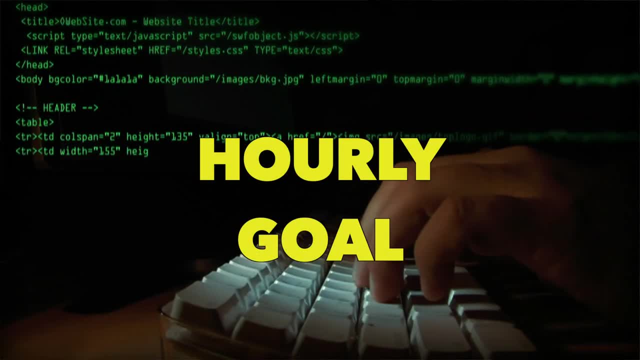 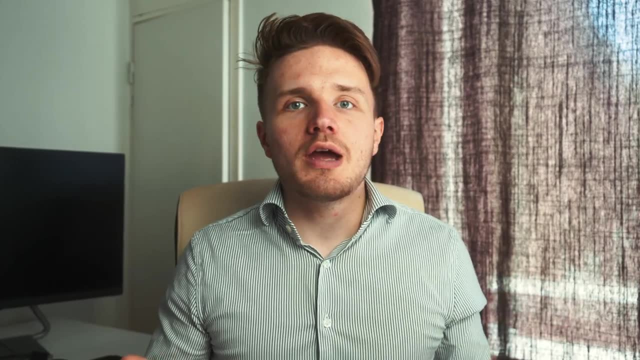 But what you need to do is set an hourly goal every single day, and how many hours you do depends on your ambition level as well as your life situation- how many hours you can do and how ambitious you are, how many hours you want to do. I would recommend, at the very least. 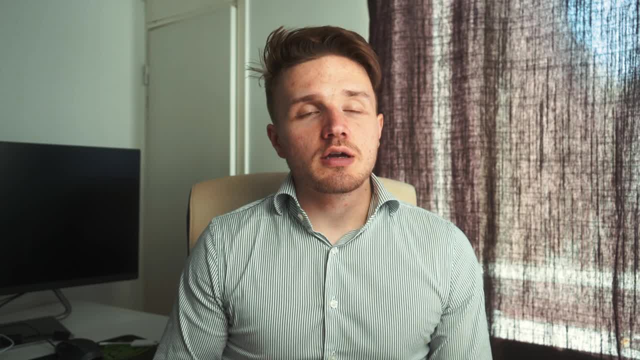 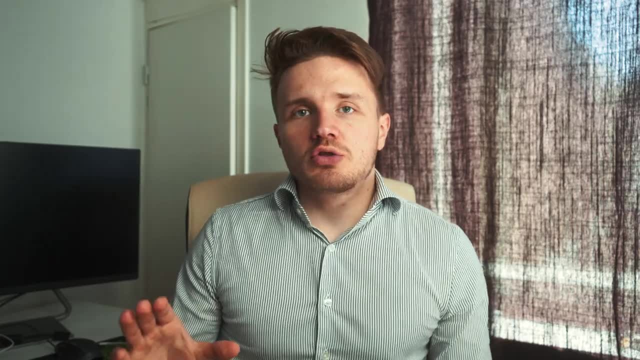 one hour every single day to get any sort of manageable progress done. Hopefully even more than that. like two to three hours would probably be good. If you're really ambitious, like I was when I was learning to code, you can do up to like five, six or even seven hours. if you don't have. 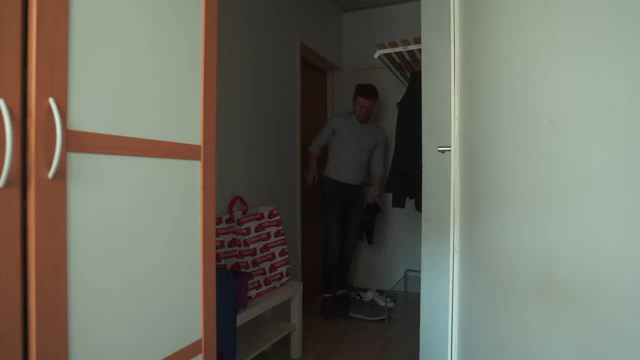 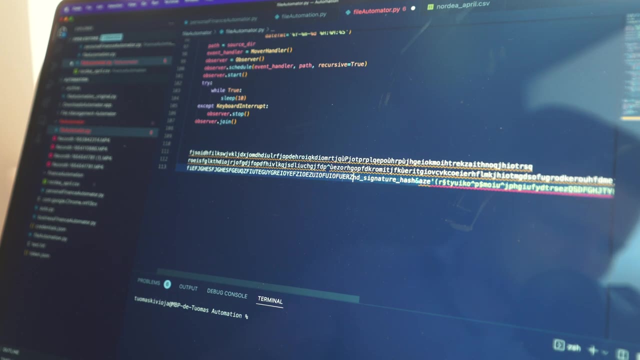 any other responsibilities. So even if you do, you can come home at 5pm, have dinner, whatever, 7pm, 10pm. you just grind coding, You just put in the work every single day and I promise you. 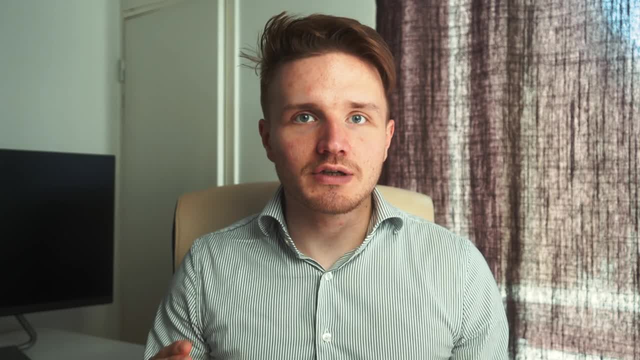 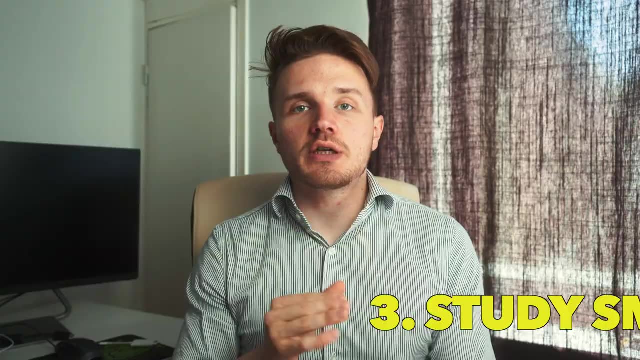 you will learn extremely fast if you just put in the hours every day. It's sort of obvious, but I feel like it just needs to be said. Number three is to not only study hard, but also study smart. Many people don't realize that not every hour that you spend studying or working is created. 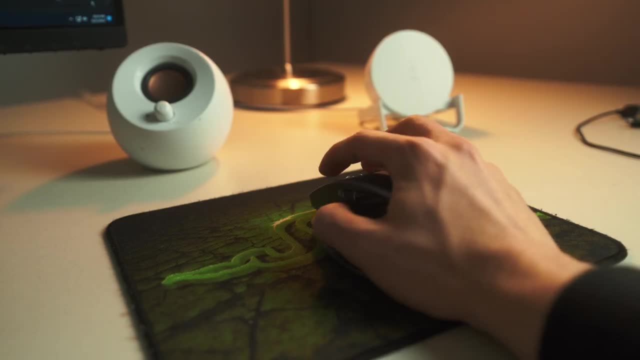 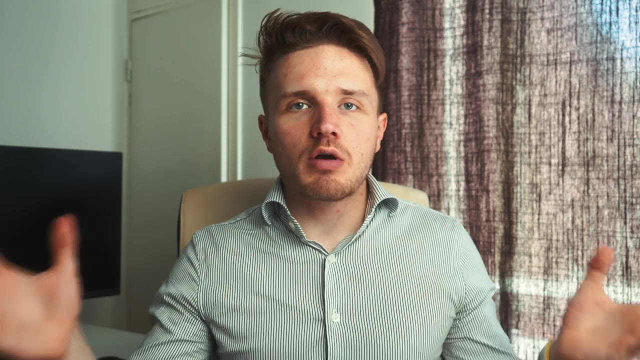 equal How effective your hours are really depending on the sort of study methods you use and how much you are able to focus during your time in your study. I made a whole detailed video around how I study smart rather than just hard, but the gist of it is that the most important. 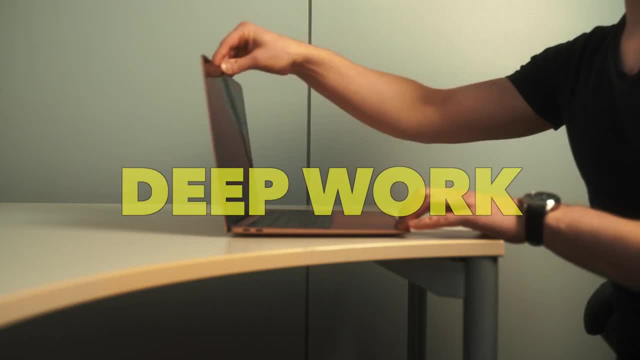 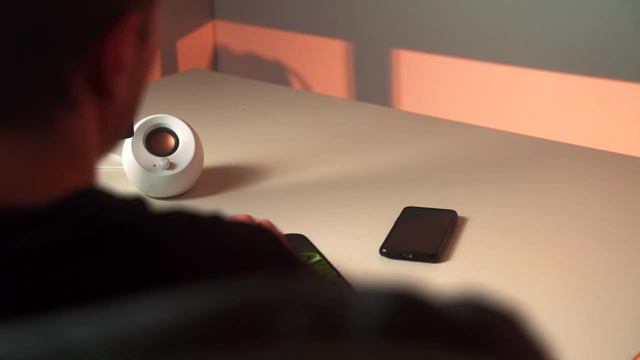 thing that you should do is start practicing something called deep work, where essentially all that means is that when you are working, you are only focused on working, You're not allowing yourself to be distracted, you don't have your phone around you, and it might seem like a very 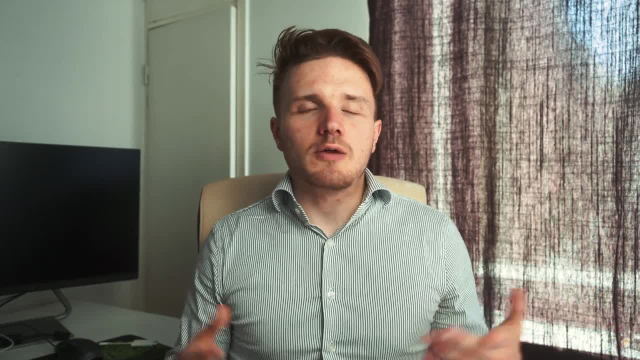 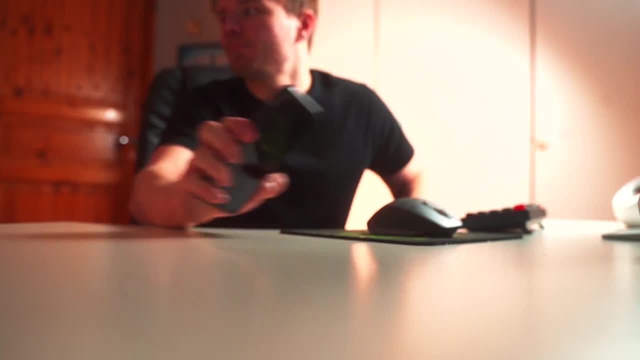 small thing, that if you get one notification that you read it like what's the big deal? That takes you back to work. But the way our brains actually work is that whenever you get out of your work, whenever you get out of your flow state, your focused state, you enter this sort of context. 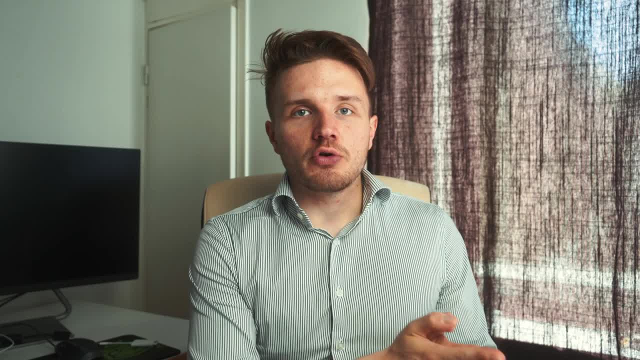 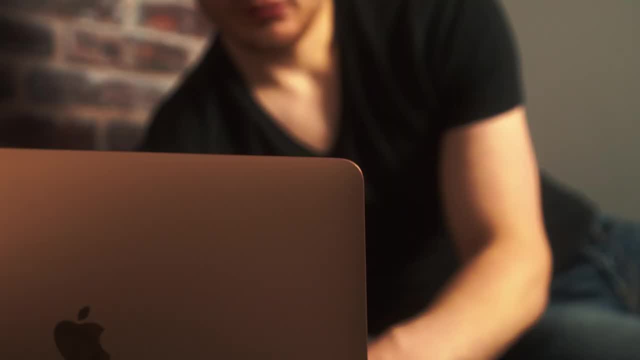 switching mode, where to get back to the same level of focus will actually take up to 20 minutes, even for a small 30 second to one minute distraction. So not being distracted is key. If you want to learn more about this, you can again watch my other videos and I'll make. 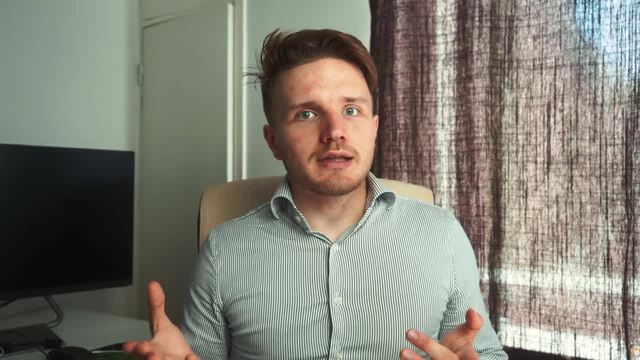 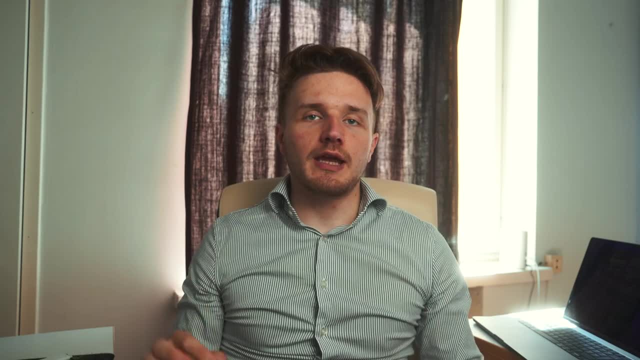 a whole detailed video on deep work if you want to see that. But yeah, study smart by implementing deep work. Last but not least, and actually most importantly, now that you've got the basics down from your basic course, which can, by the way,